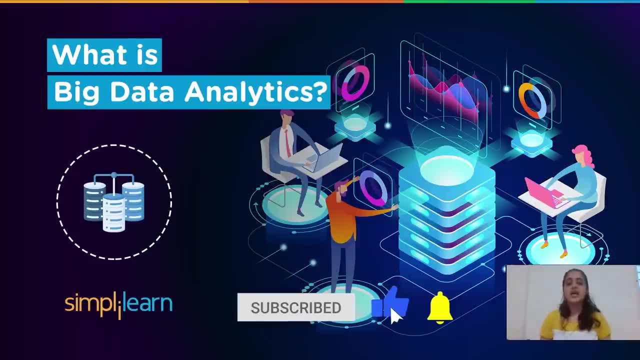 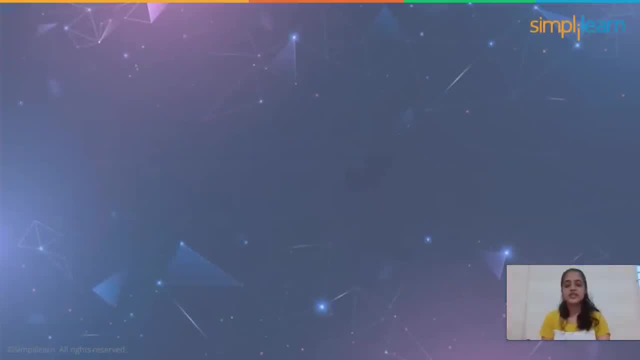 we start, please make sure you subscribe to our channel and press the bell icon to never miss an update. So let's go through the topics to be covered in today's video. Let's start by getting introduced to what is big data analytics. Next we will learn about 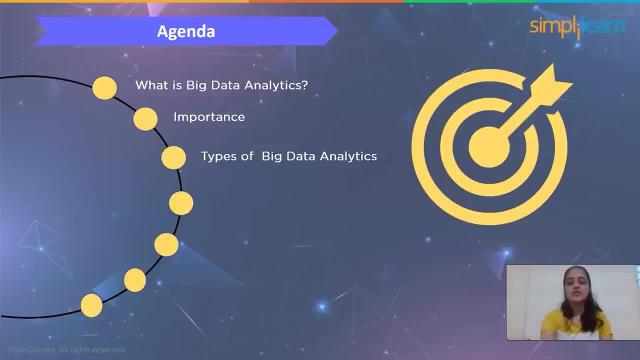 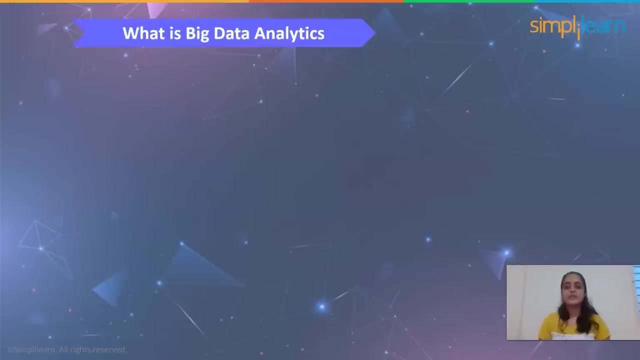 importance of big data analytics, Next types of big data analytics, followed by life cycle of big data analytics, tools and advantages of big data analytics and finally, we will go through use cases of big data analytics. First, we must understand what do you mean by big data analytics? Big data analytics is the technique to analyze. 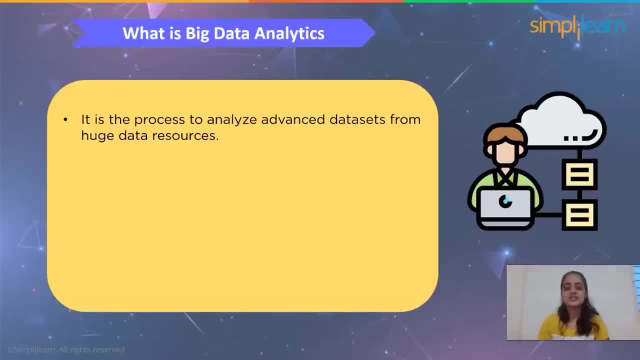 valuable data sets having any format, like structured, unstructured or semi-structured, For example, music industries like Spotify. The company has nearly 96 million users that generate tremendous amount of data every day Using this information. the application generates a huge amount of data every day, For example: the company has nearly 96 million users that generate tremendous amount of data every day Using this information. the application generates a huge amount of data every day. For example, the company has nearly 96 million users that generate tremendous amount of data every day Through: 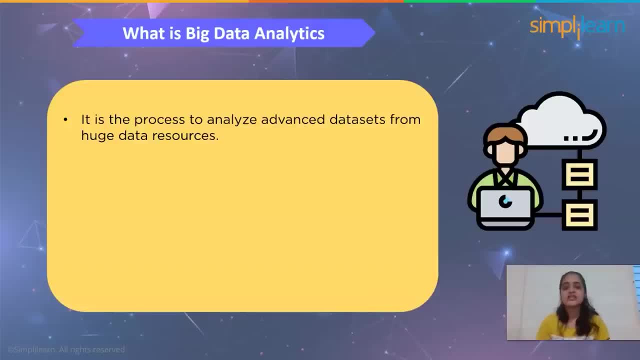 Naakes, SuggestiveScans, Likes, Shares, Paying Comments and other services. the locals are using it for creating TikTok behaviour. Also, some is: you shouldn't do such things. you are just marketing them for their institutions to achieve high success rates in today's data analytics platforms. 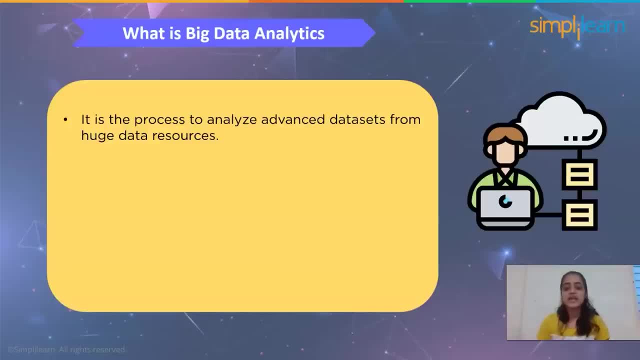 Playlists are created automatically and many more automated processes can happen to you. What enables this are the techniques, tools and frameworks that are a result of Big Data Analytics. If you are a Spotify user, then you must anyway have come across the top recommendations. 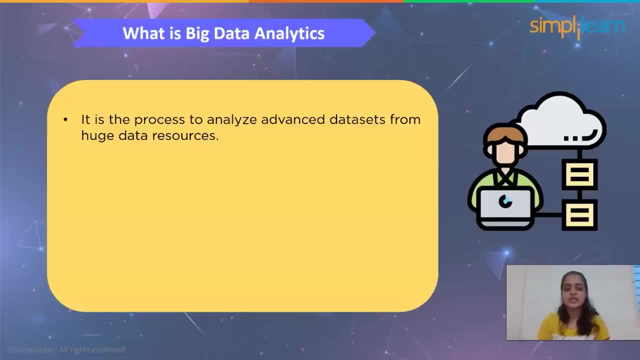 section, which is based on your likes, past hits and other things. Utilising a resource that isaced on No poll last day, we get easily an leadership in the game parlour of for everyone, especially on customers from —for people who our recommendation engine that leverages data filtering tools that collect data. 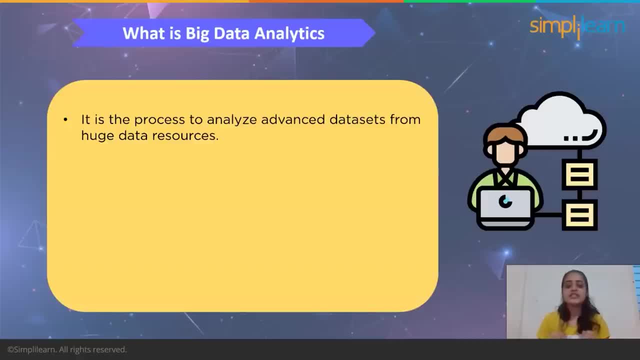 and then filter it using algorithm. this is how Spotify works, by collecting and analyzing proper data and incorporating it into business plans, which will further help them in decision-making. this is how the data analytics helps big business organizations. seventy two percent of e-commerce companies rely on data produced from 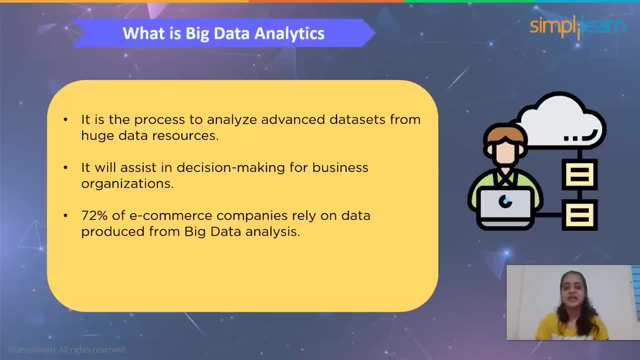 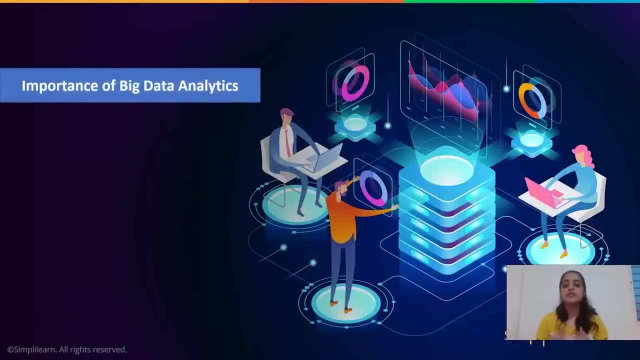 big data analytics, and this data is increasing day by day. any YouTube channel can use data analytics to analyze user interest and develop his next project based on that. what is the importance of the topic? why do we need to study big data analytics is the biggest question. it is observed that 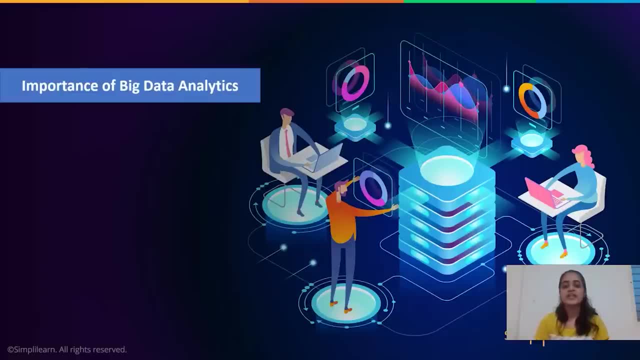 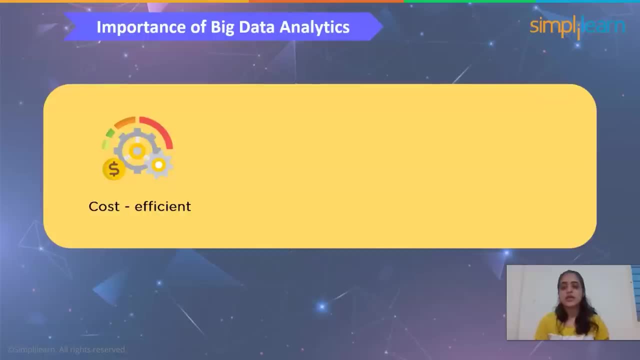 every organization adopts this technique for better understanding of data and its use. cloud-based analytics can store a large amount of data with minimal cost. for example, tools like Zoho analytics, Microsoft power bi and manimo does big data analytics can result as cost efficient. the way of analyzing it is very Swift, which will help to analyze. 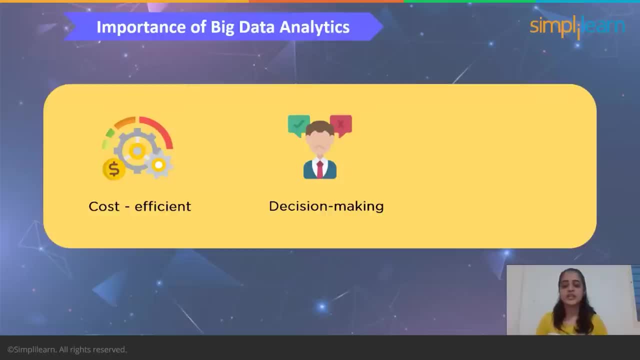 all the sources. this is how big data analytics. This will contribute to quick decision making in any organization. The result of such analysis will help to develop new products As, due to these products, analysis of the companies will know about their customer likings and behavior. 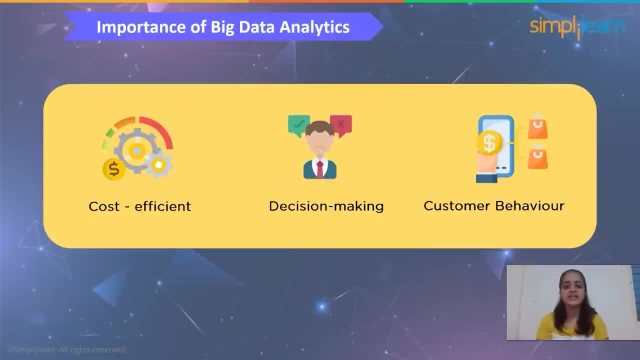 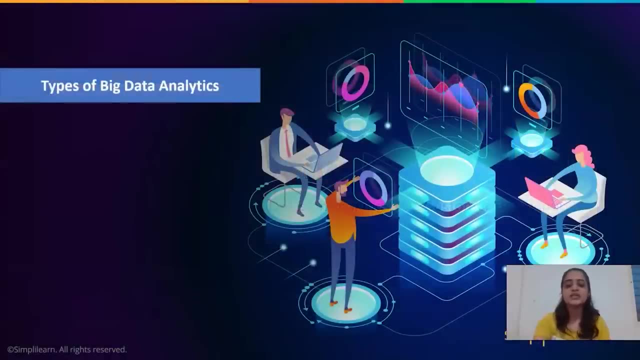 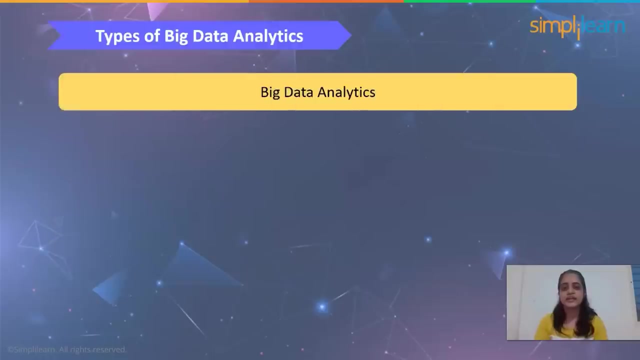 Due to all these efficient strategies, big data analytics is very crucial. Let's move forward and understand what are the types in big data analytics. First, let's try and understand descriptive analysis. It includes processing past and present data set, which will lead to help in trend analysis. 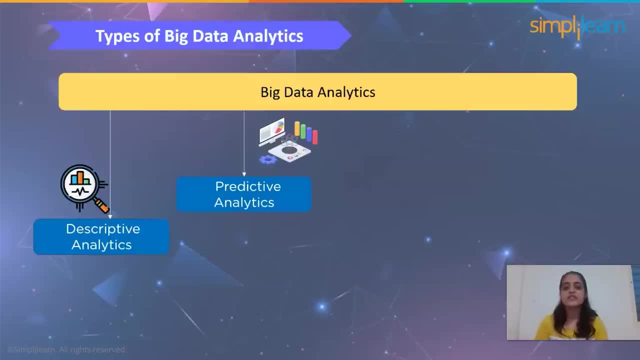 In predictive analysis. it makes future predictions based on past or historical data sets and which will help in decision making. The Diagnostic analysis is an advanced analysis system in which introspections are made based on why that has happened and further decisions are taken based on the available data sets. 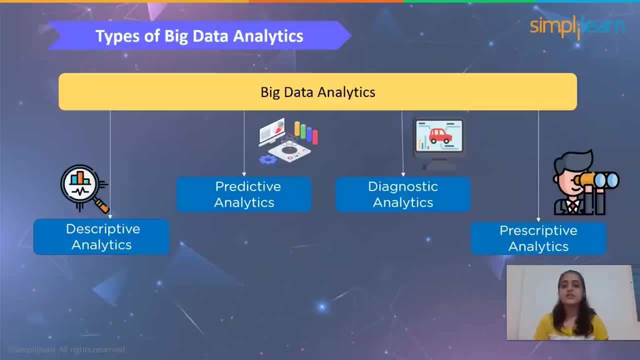 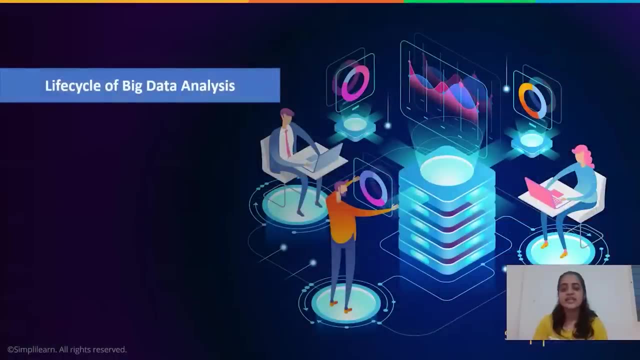 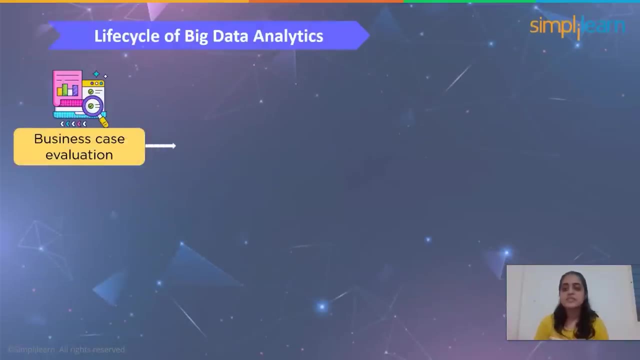 Prescriptive analytics is the process of using data to determine an optimal course of action. The next topic we are covering is Life Cycle of Data Analytics. First is business case evaluation will help decision makers to understand the source of business. In this case, the learner or the team will learn about the business domain which presents. 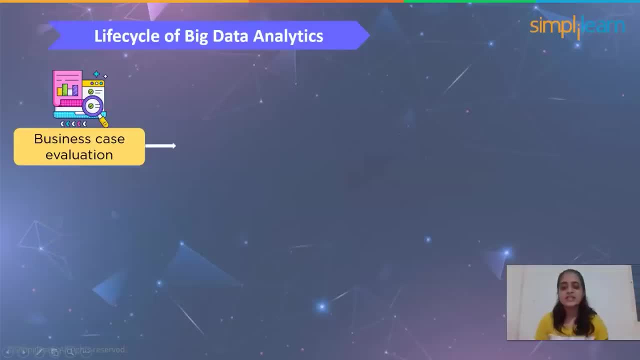 the motivation and goals for carrying out the analysis. In this point, the problems get identified and assumptions are made based on the available data sets. In this case, the learner or the team will learn about the business domain which presents the motivation and goals for carrying out the analysis. 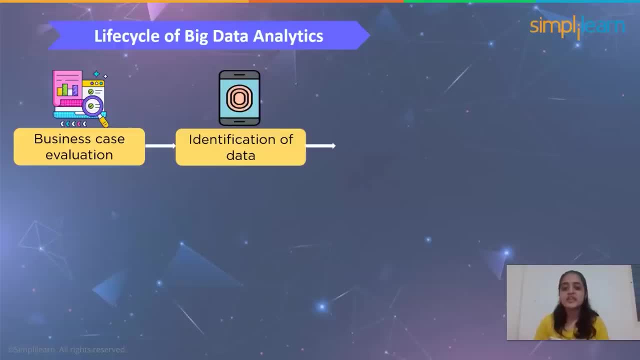 In the identification of data. once the business case is identified, now it's time to find the appropriate data sets to work with. In this stage, analysis is done to see what other companies have done for similar data sets In data filtration. once the source of data is identified, now it's time to gather data. 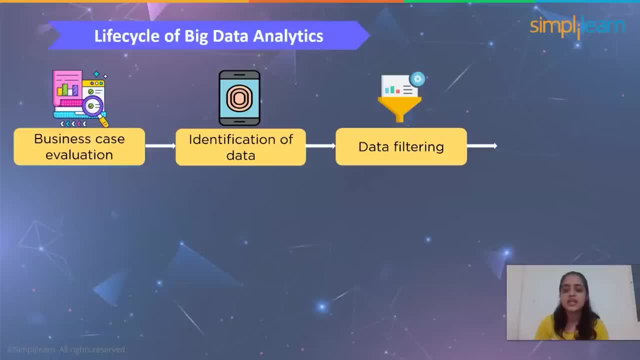 from such resources. This kind of data is called data filtering. This kind of data is mostly unstructured. Then it is subjected to filtration, such as removal of corrupt data or irrelevant data which is of no scope further. Then it is subjected to filtration, such as removal of corrupt data or irrelevant data. 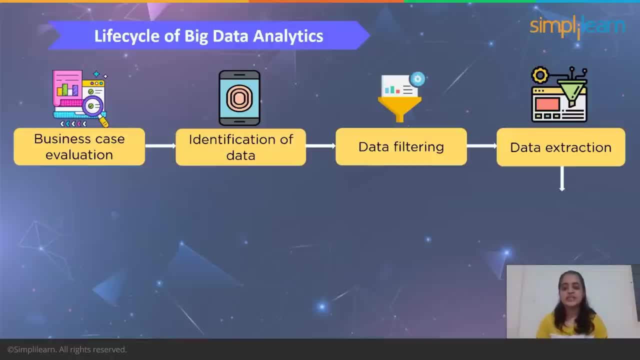 which is of no scope further. Now the data is filtered, but there might be a possibility that some of the entries of such data is incompatible. To rectify this issue, a separate phase is created, called as extraction phase. In this phase, the data which don't match the underlying scope of the analysis are extracted. 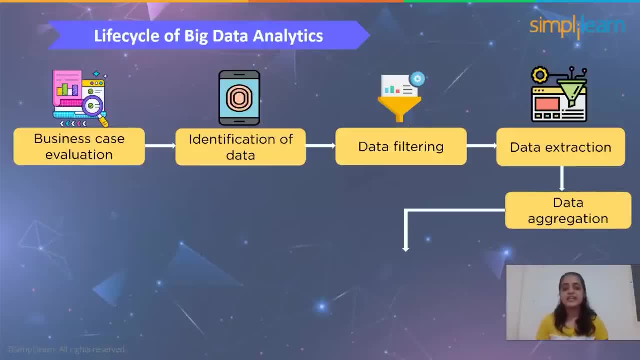 and transformed In data aggregations. datasets are validated and combined with common field. For instance, we can take dataset of a student. One dataset can be named as student academic section and the other can be named as student personal details. Then both can be joined. 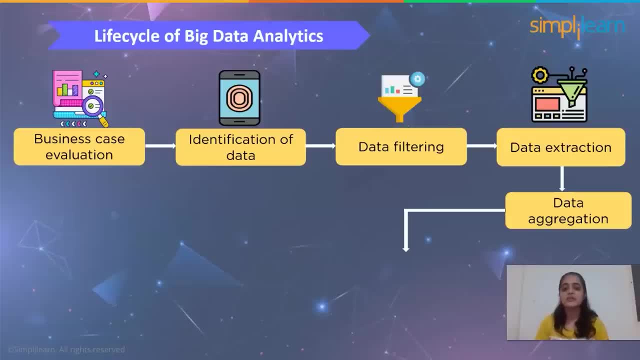 together via common field. We can take it as roll number. Depending on the nature of big data, problem analysis is carried out. Data analysis can be classified as confirmatory analysis and exploratory analysis. In confirmatory analysis, the cause of the phenomenon is analyzed. 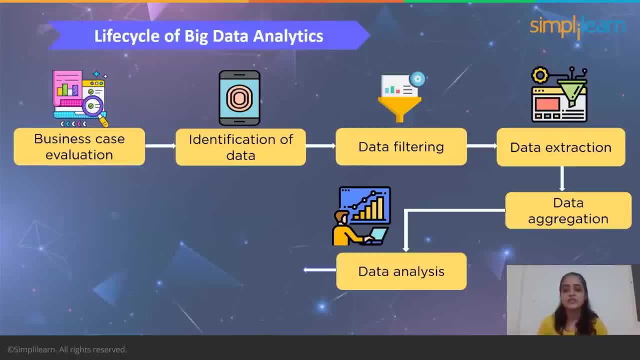 before The assumption is called hypothesis, The data is analyzed to approve or disapprove the hypothesis. Such kind of analysis will provide definitive answer to some specific questions and confirms whether an assumption was true or not. In exploratory analysis, the data is explored to obtain information that why a phenomenon? 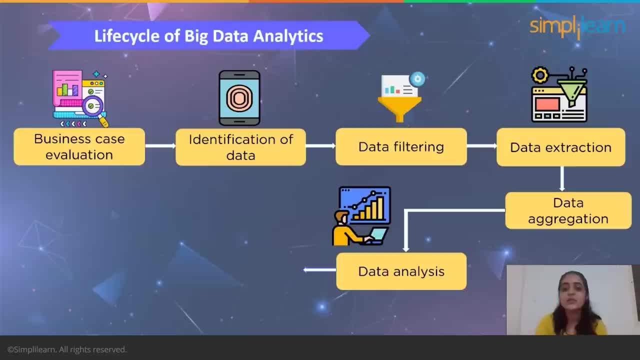 has occurred, This type of analysis answer why a phenomenon occurred? This kind of analysis doesn't provide definitive information. Meanwhile, it can provide discovery of certain patterns. Visualization, or data visualization, is said to influence the interpretation of the results. Moreover, it will allow the user to discover answers to the question. 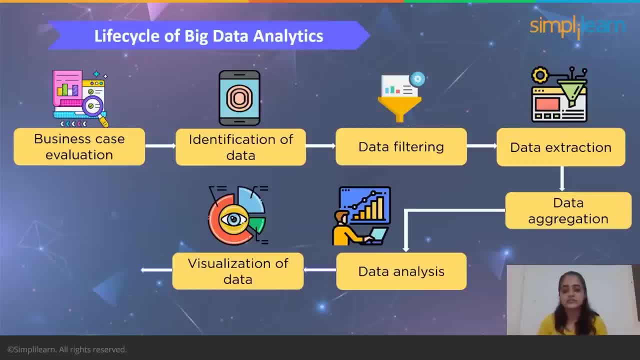 The analysis is done. The results are visualized. Now it's time for the business user to make decisions using the result. The result can be used for optimization, to define business processes. It can be used as an input for the system to enhance performance. 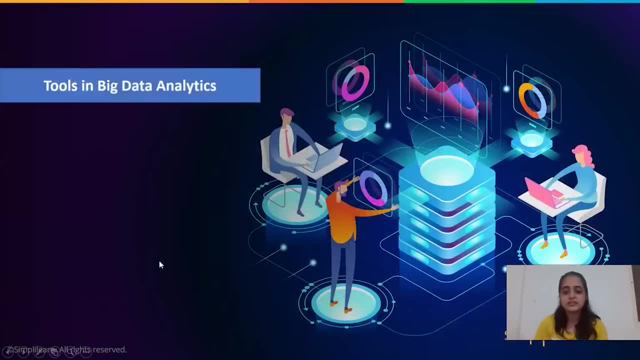 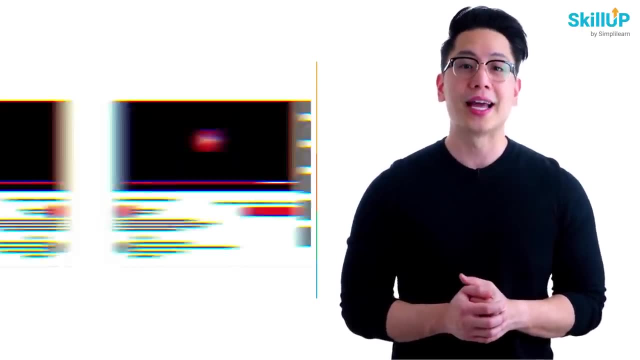 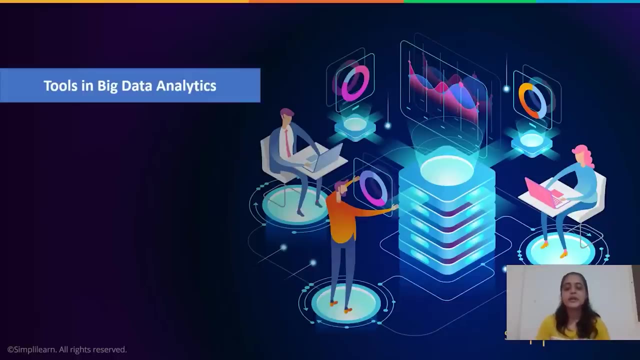 This is all about lifecycle of data analytics. If getting your learning started is half the battle, what if you could do that for free? Visit ScaleUp by SimplyLearn. Click on the link in the description to know more. There are multiple tools available on the market which can help companies in big data. 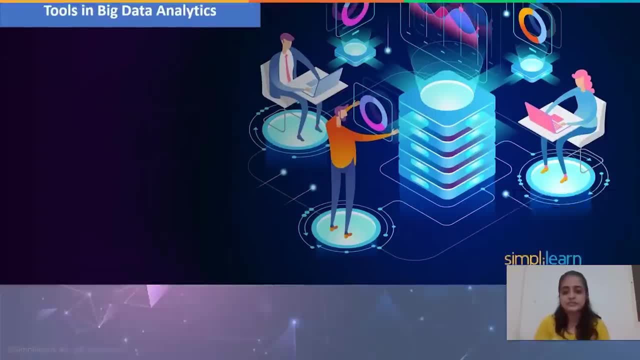 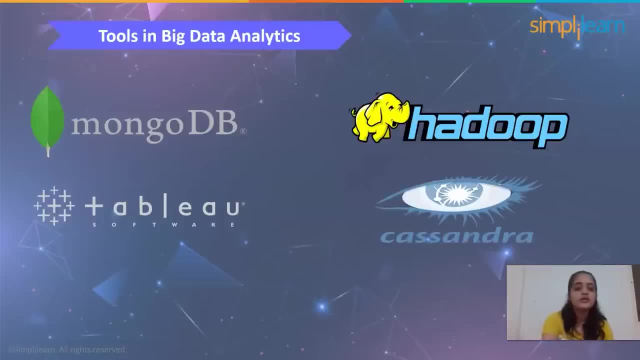 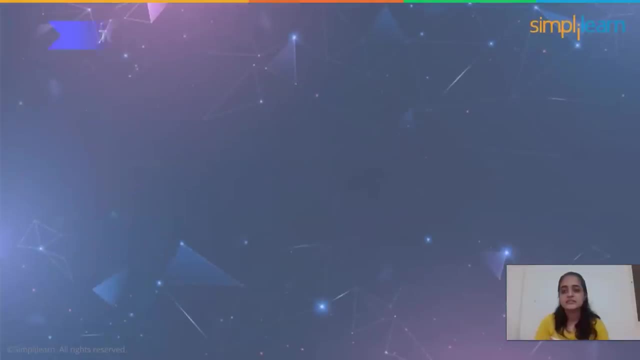 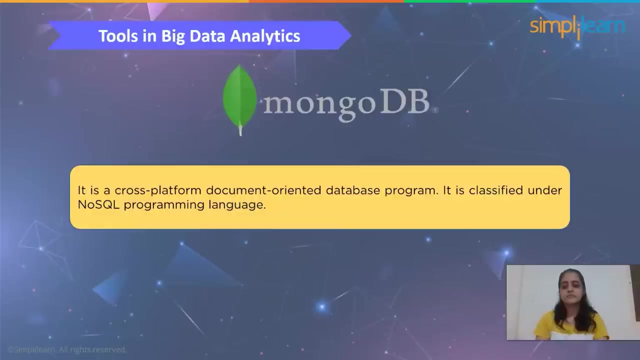 analytics. Let us go through some of these tools: MongoDB, Hadoop, Tableau, Cassandra. These are the main tools which are used to create big data analytics. Let's go for MongoDB. MongoDB is an open-source tool that supports data storage. It is a no-SQL, document-oriented. 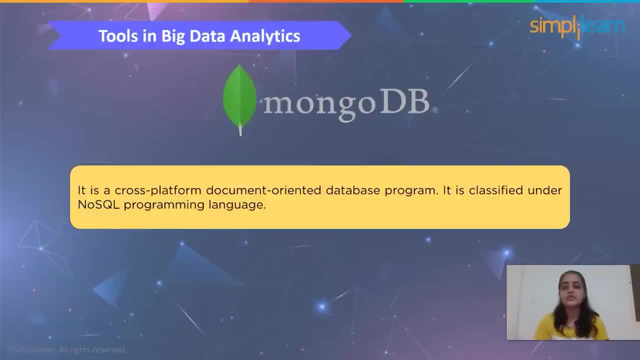 database. MongoDB is used by Facebook and Google for data storage. MongoDB is best suited for big data, where resulting data and further manipulations can be done. It can be used for data storage. It can be used for data storage. It can be used for data storage. It can be used for. 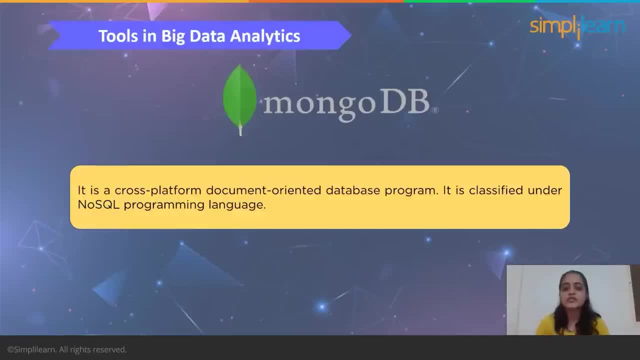 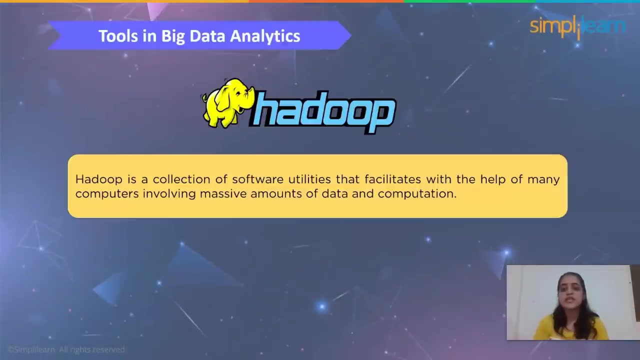 100 days For this. theணes of information can be used to create big data analytics. Some of the powerful resources are grid operations, aggregation, framework text, research and the map produce features. Apache Hadoop is the most famous tool. It is an open-source software utility to store. 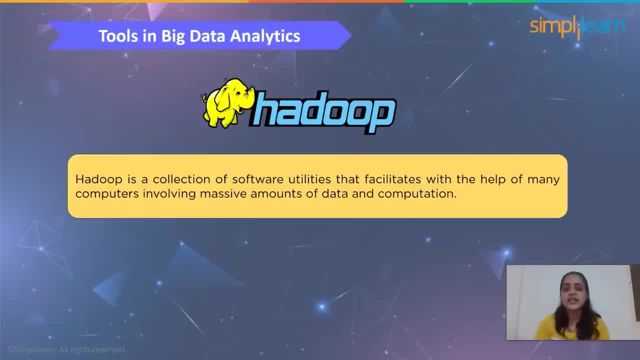 and process gigabytes and terabytes of data. It uses the map reduce programming module to solve problems of anything analyzing massive data. MapReduce is a framework that helps programs do the parallel computation on data. The map task takes input data and converts it into a dataset. 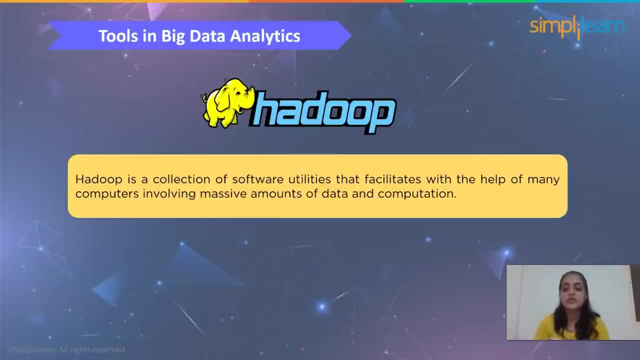 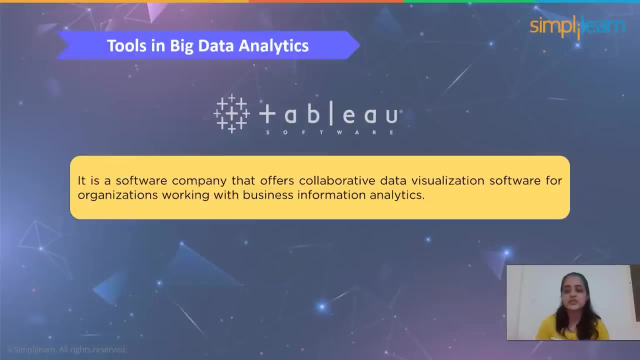 that can be computed in key-value pace. The output of the map task is consumed by reducing tasks to aggregate output and provide the desired result. Tableau is a software company that offers collaborative data visualization software for organizing working with business. information analytics Organizations use Tableau to visualize data. 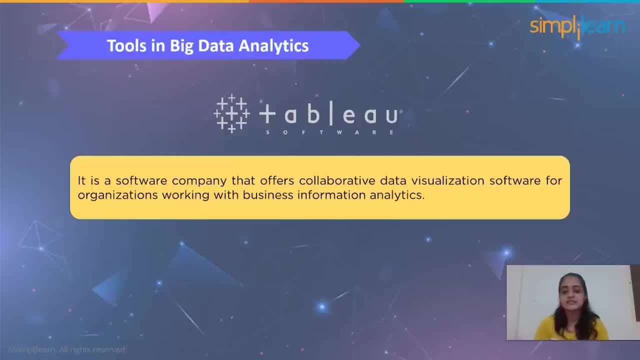 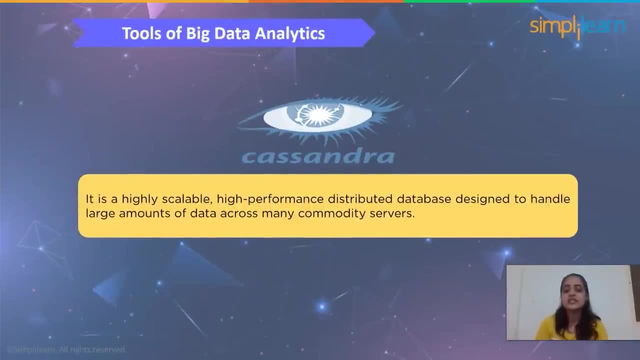 and reveal pattern for analysis in business intelligence. Apache Cassandra is highly scalable, high-performed distributed database design to handle large-end data. It has a large amount of data across many commodities, like servers, providing high availability with no single point of failure. It is a type of NoSQL database. 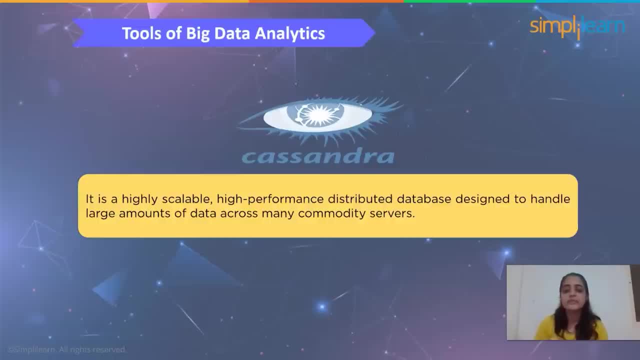 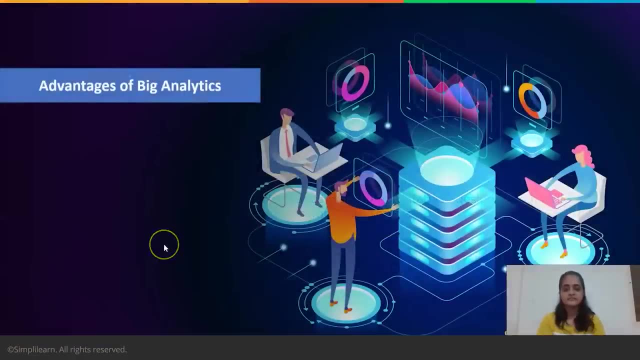 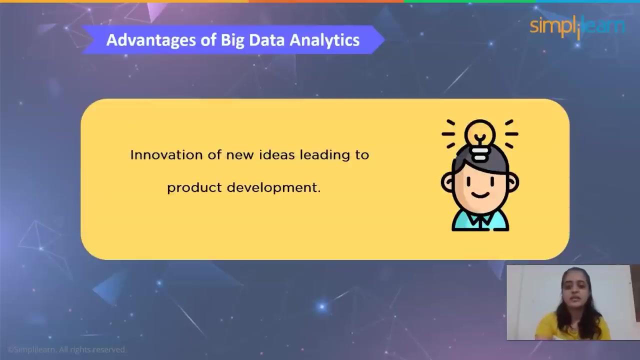 Now we have covered the important tools used by big data analytics, Let us go and cover distinct advantage of big data technology. Advantages of big data analytics: Innovation of new ideas leading to product development, which means developing new products, provides a means to target new markets, increase market share, sell more. 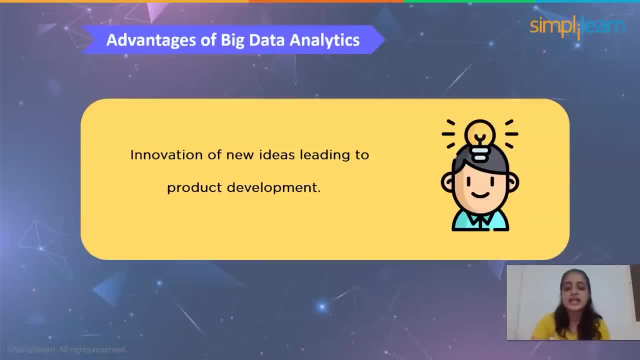 and increase revenue streams. Meanwhile, redesigning existing products enables cost to be cut, margins to be decreased and, ultimately, more profits to be made. Risk management insights about customers likings and behavior and market trends will help decision maker to take their position. 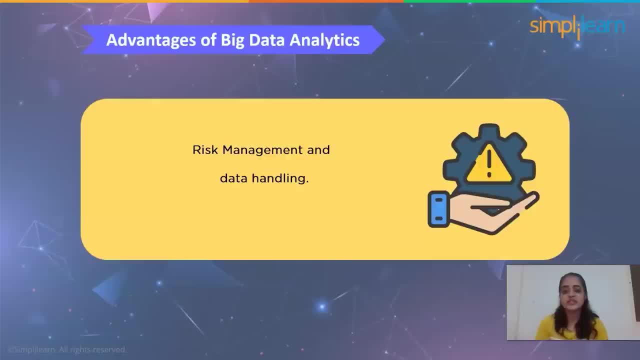 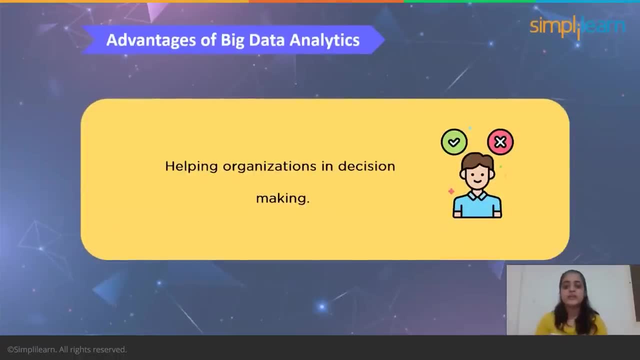 On top of that, it will help to get rid of financial risk. It will also assist to detect potential cyber risk. One benefit from big data and business analytics can help improve decision making by identifying patterns, Identifying problems and providing data to back up the solution is beneficial. 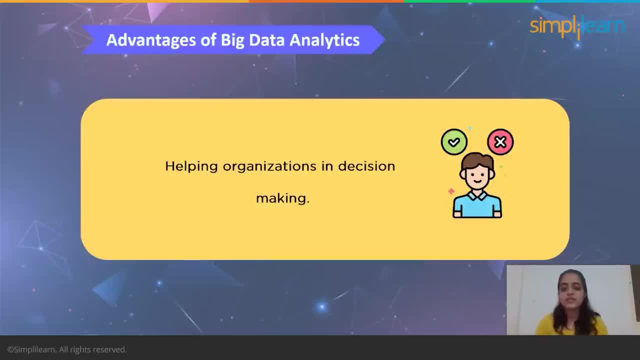 Whether the solution is solving the problem, improving the situation, or it has an insignificant effect. Here, customer engagement, specifically how your customers view and interact with your brand, is a key factor. Big data analytics provides the business intelligence you need to bring about positive changes. 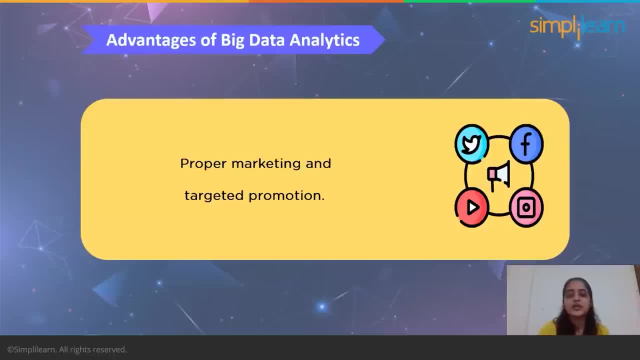 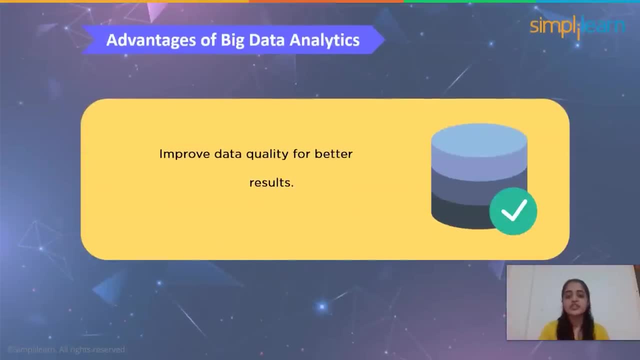 like improving existing products or increasing revenue per customer. Next, improving data quality will improve your business. Next, improving data quality will improve your business. Next, improving data quality will improve your business will improve operational efficiency and valued feedback from customers, which will help businesses. 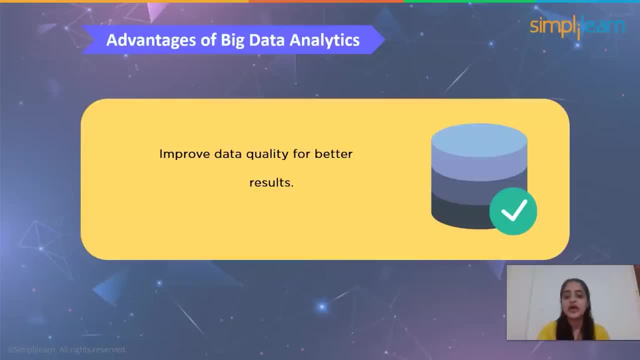 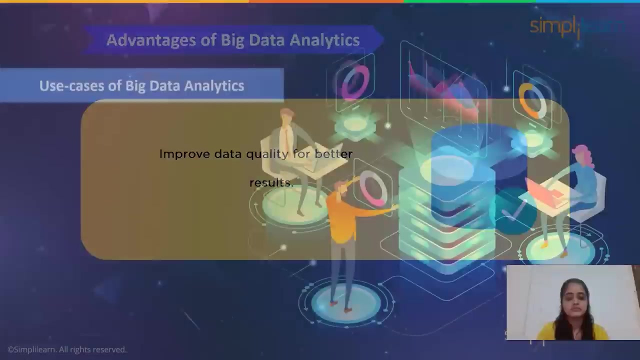 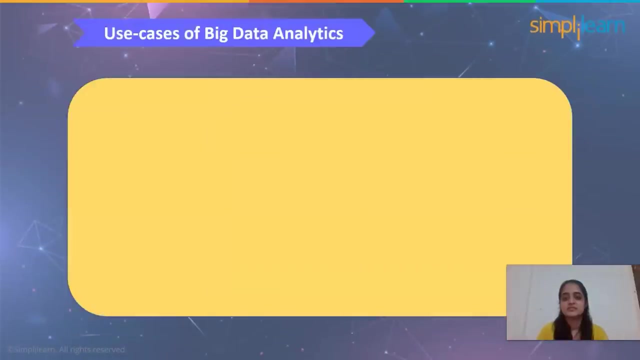 to handle vast amounts of data. It will also help in enabling data-driven decisions. But how do these advantages related to the real world? Let us cover some real-life use cases empowered by Big Data Analytics. Use Cases of Big Data Analytics. Amazon is a well-known name to all of us. It is among the leading e-commerce platforms. 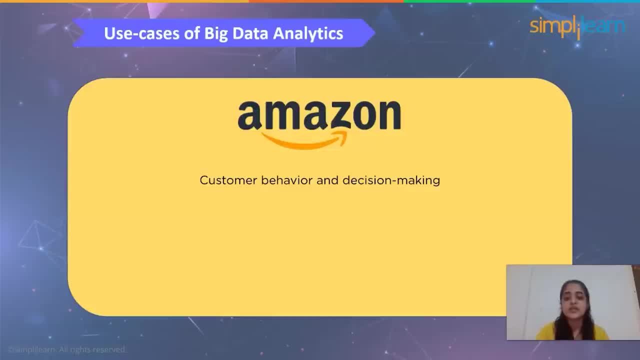 Apart from offering online shopping, Amazon serves us with different services like Amazon Pay, Amazon Web Services and many more. For a company like Amazon, the amount of data collected on a regular basis is very big. To manage such vast amounts of data, 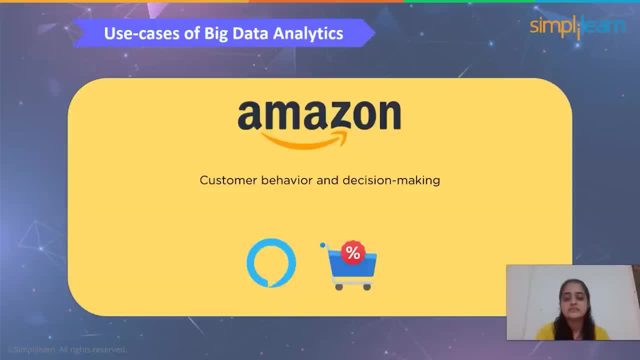 companies leverage big data. For any company like Netflix, one of the most valuable assets is the customer base, because it is the customer who turns the company into a brand, And if a company fails to meet the expectations of the customer, that probably leads to its decline. Big data is a technology that helps in the management of large 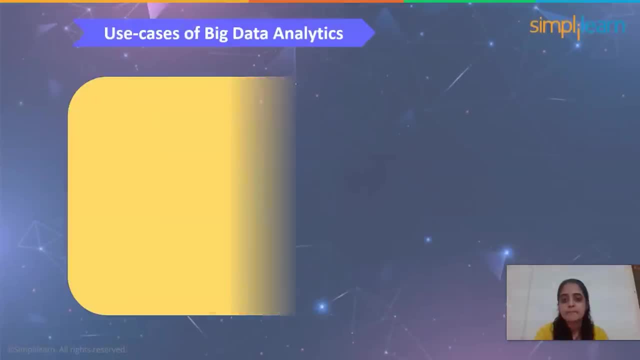 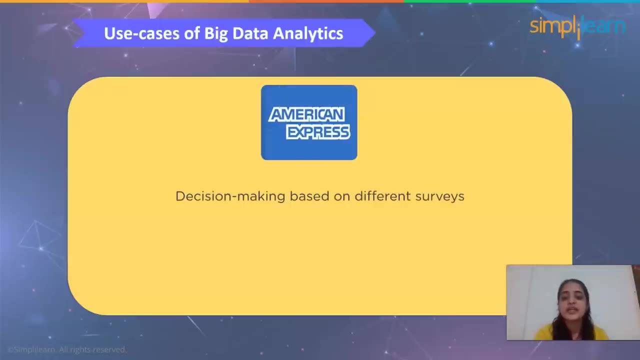 data. Big data is like a heart for American Express decision making. Their main goal is to detect fraudulent transactions as soon as possible for reducing loss, and in this big data plays a very important role. They use big data for anticipating and analyzing customers' data.